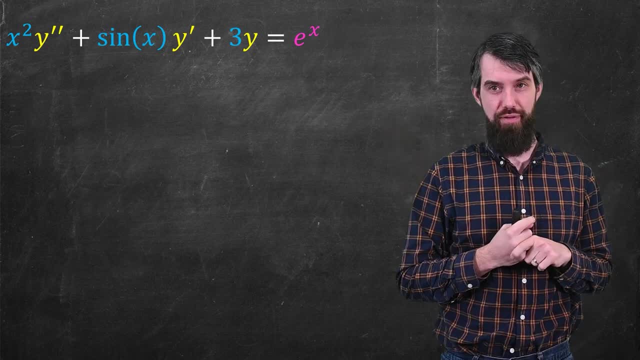 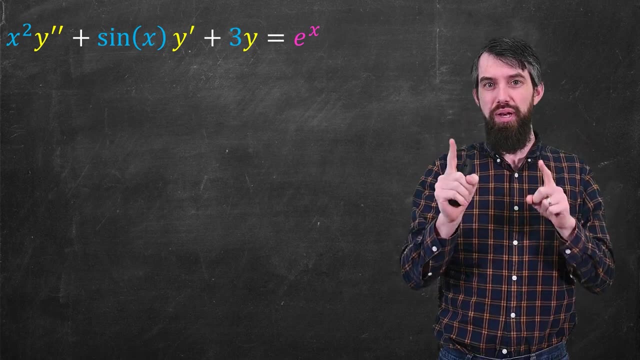 linear differential equation. Well, this is an example of it and it looks quite messy here. I mean, there's lots of squared terms, there's a sine of x term, there's an exponential term. But notice the following very important fact: The function y, the function y prime and the function y double prime. 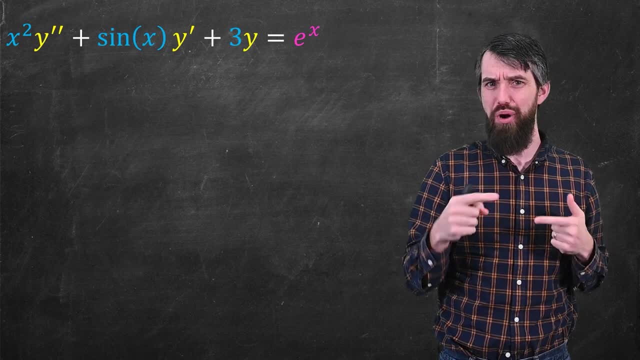 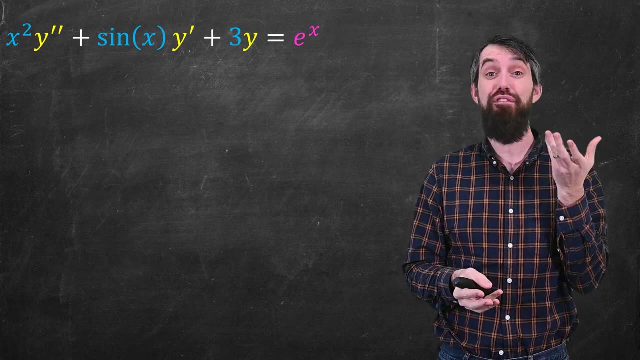 all of those are what we're going to call linear. It's not like it's y prime squared or e to the y. The y prime just sits by itself to the power of one and is multiplied by a coefficient function. So the coefficient function of y double prime. 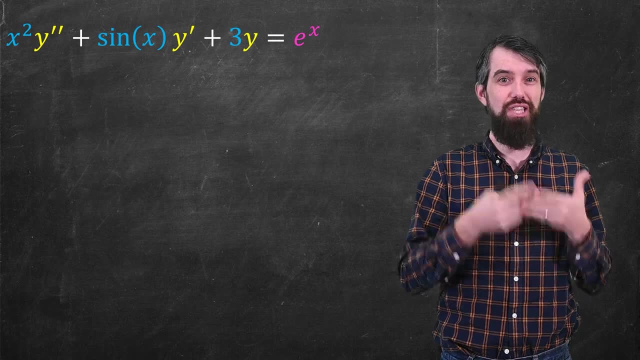 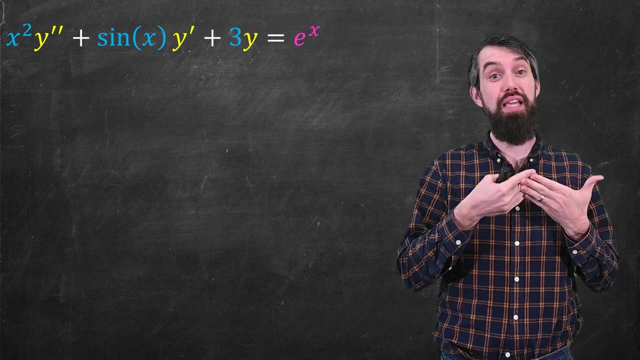 was x squared, The coefficient function of y prime was sine of x. The coefficient function of y was three and, if you like to think of it this way, the coefficient function of just one was e to the x. So this is an example of a linear second order, because there's two derivatives. 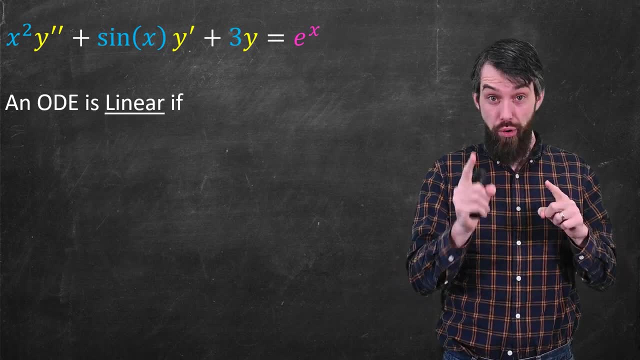 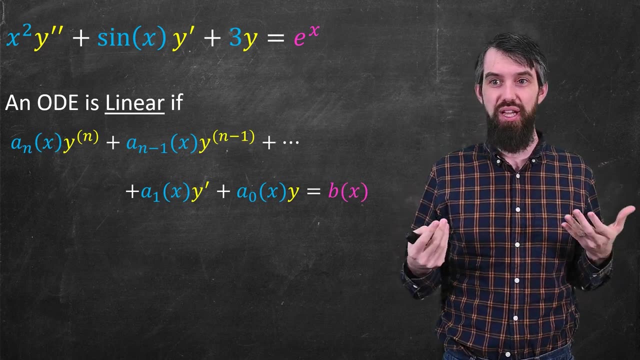 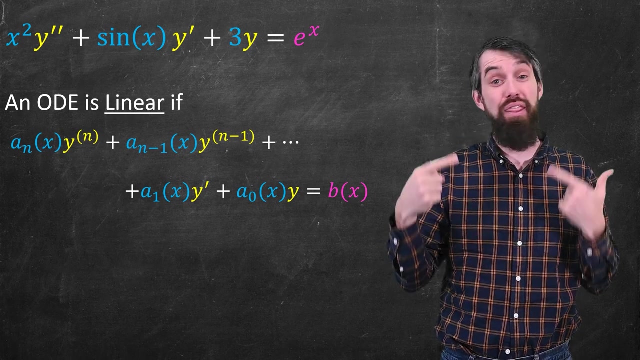 differential equation, More generally a ODE. an ordinary differential equation is called linear if it obeys the following property: It's just a bunch of derivatives. y, y, prime. all the the times is just a bunch is a bunch because this is what it's called a basical exponent solution. 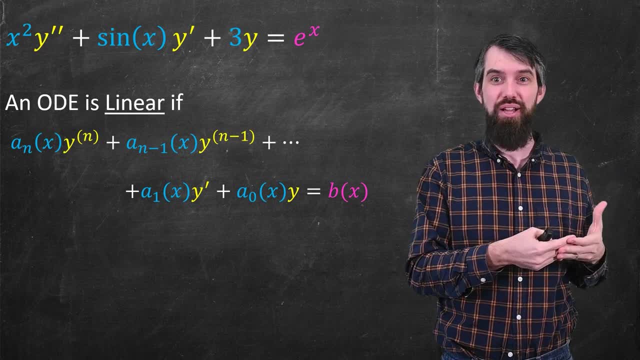 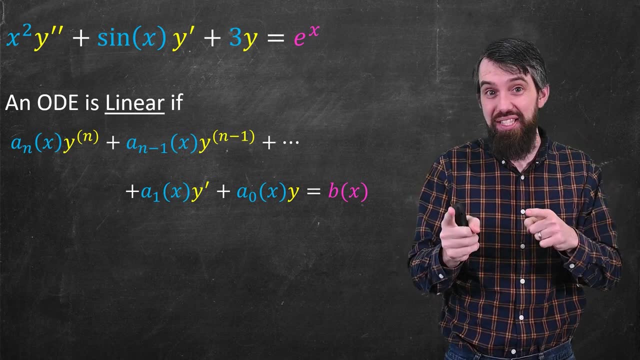 You may have noticed this before editing the video, Dean. let's say, for example, if i flinched five times and you의d like to have your own вал with noakers on it, relating that teża, then i. what can you think of it? 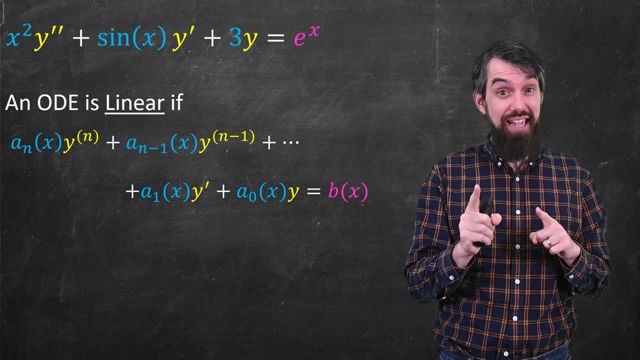 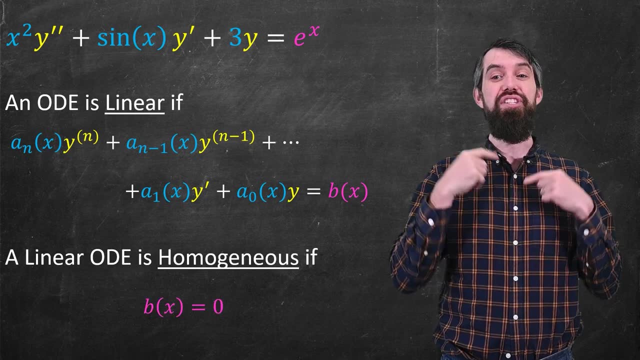 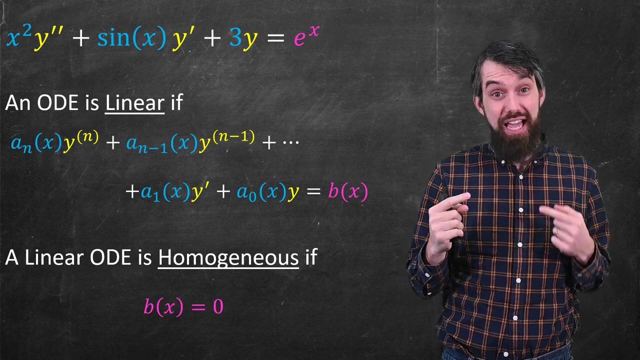 Gradually it would rise to a larger joule. then you get a simple, better thing for all. a勿톱 function 1, no y's at all If that is 0, we additionally call it a homogeneous linear, ordinary differential equation. Now, if you've taken linear algebra- and it's okay if you- 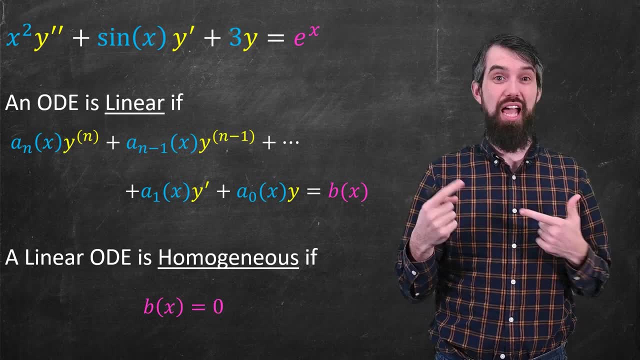 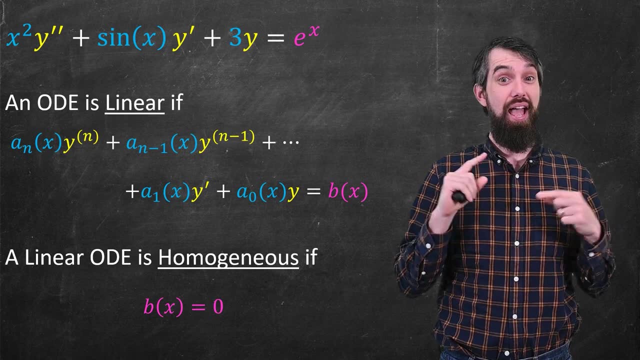 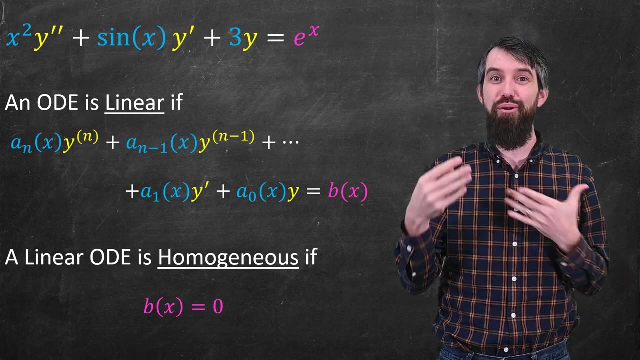 haven't, then you've seen these types of terms before. For example, if you had a linear equation, it might represent, for example, a line or a plane. And if that linear equation was additionally a homogeneous linear equation, so there was no constant term, it'd be a line or a plane. 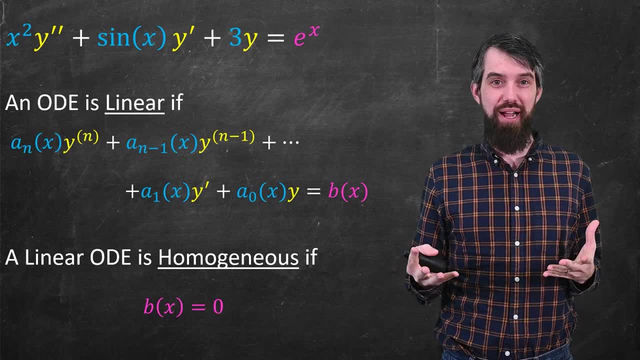 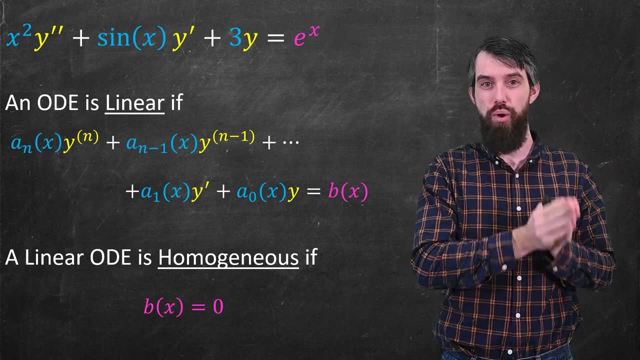 through the origin And we had this whole theory of linear algebra, which was really well developed because we love linear equations as opposed to nonlinear equations, which we still love but are a little bit more challenging. And while there's no derivatives in linear 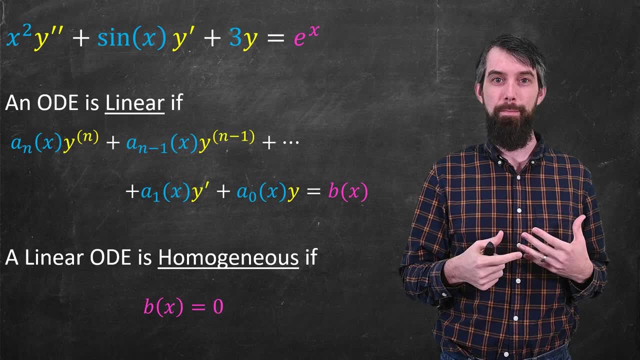 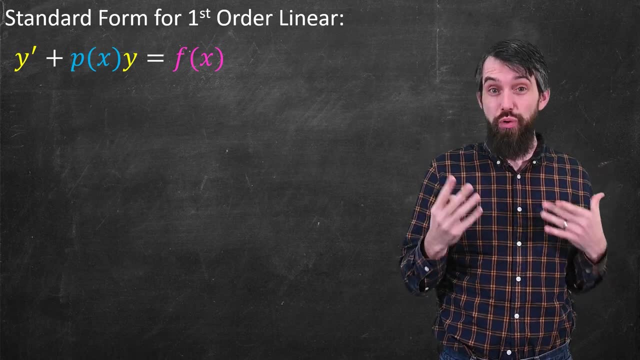 algebra. a lot of that metaphor is going to be true here as well. Now in this video we're really going to focus on first-order linear differential equations. have a method called the integrating factor method to be able to do that. 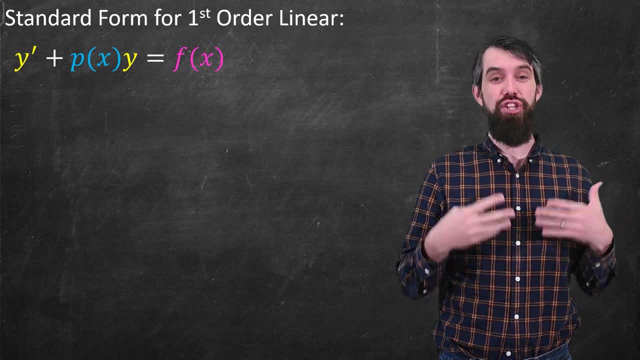 Now in this video we're really going to focus on first-order linear differential equations, have a method called the integrating factor method to be able to do that. So the first thing I'm going to do is write down a generic first-order linear, ordinary differential equation. 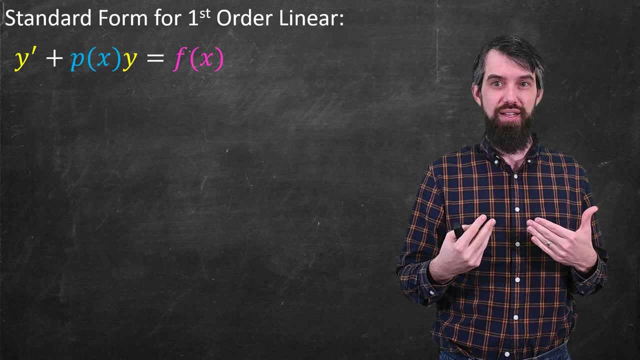 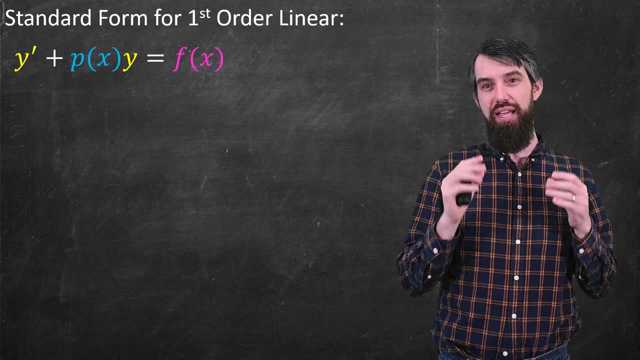 it's a mouthful in what we're going to call its standard form. So the standard form is a little bit of a different notation than what I just introduced with the a? n and the a? n minus one and so forth. In the standard form for a first-order it goes y prime, which. 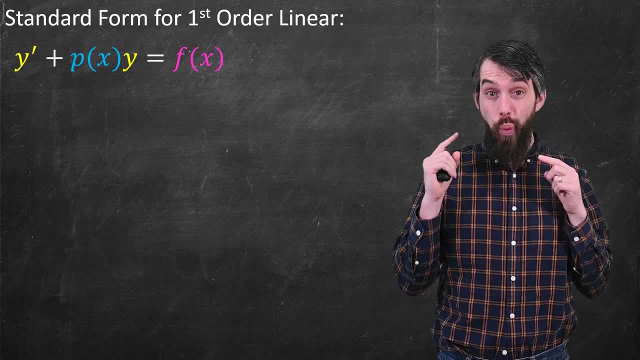 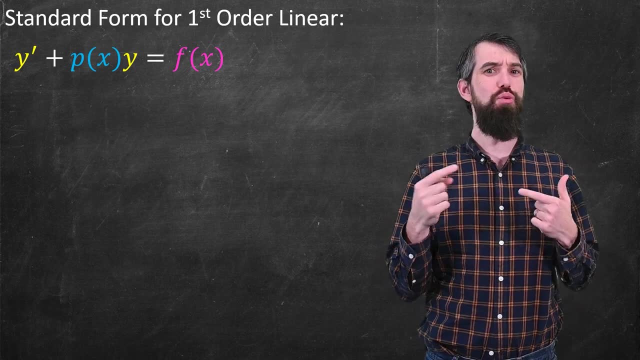 is basically saying a coefficient function of one. then y gets multiplied by p of x, so the coefficient function of y. Then on the right-hand side you have this f of x. If you ever had it written in the previous form, where there was also a coefficient function in front of the y prime, you would. 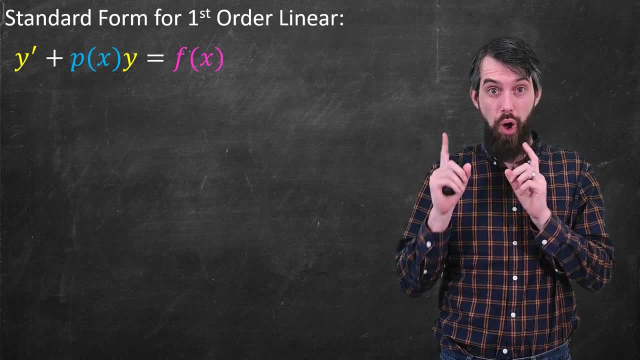 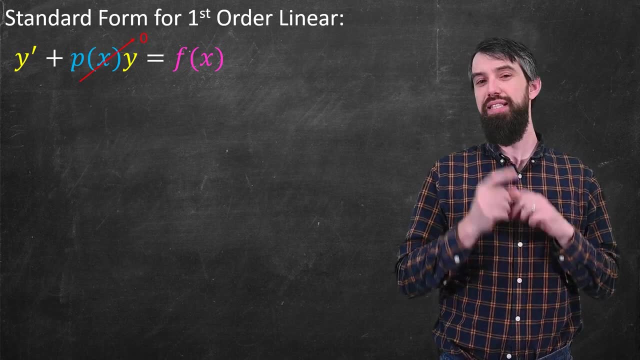 just divide it out to get your p of x and your f of x. Okay, so that's the form, but how can I solve this Now? I want you to imagine something. Imagine it was the case that p of x was equal to zero. If p of x was equal to zero, then 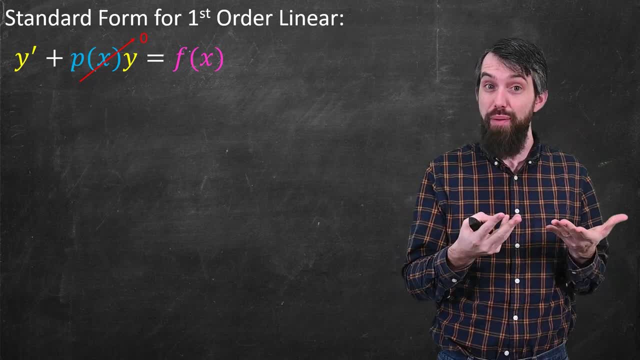 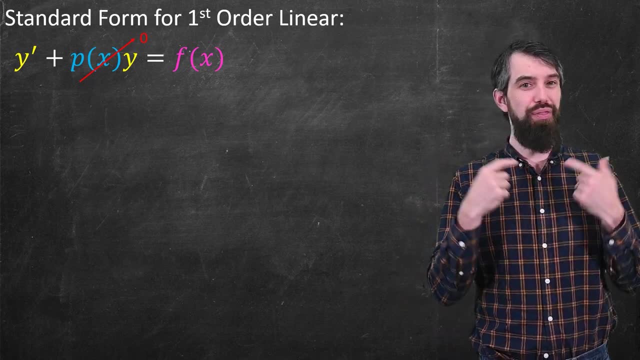 I think you could solve this differential equation. You'd just have y prime on the left, you'd have f of x on the right. You could just integrate. A derivative is a function. You could just integrate and get the answer. That is, if ever your differential equation is just written as a derivative by: 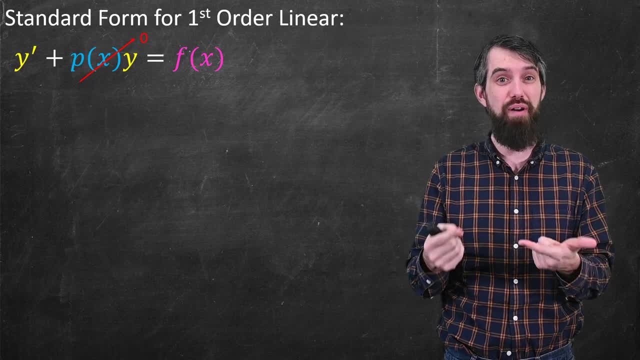 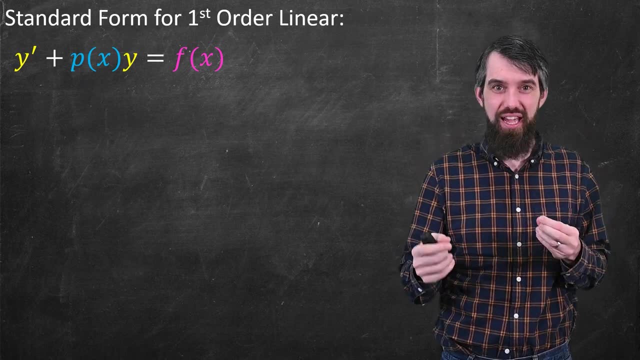 itself is just equal to the function of the independent variable, then it's easy: You just integrate. But we don't have the fact that p of x is equal to zero and we're sort of going to try and fake it by a method called the method of integrating factors. So here's how it works. 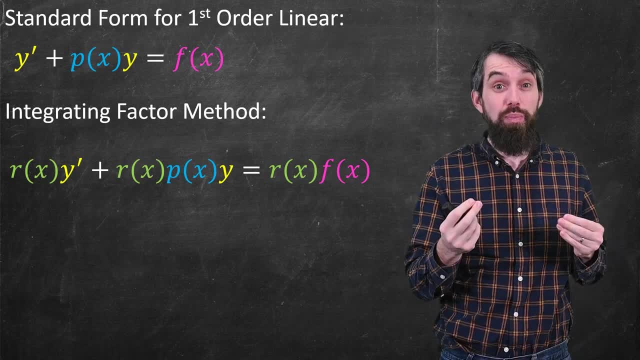 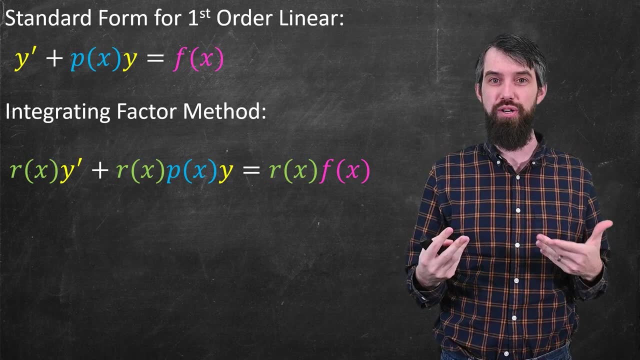 I'm going to take the same differential equation but I'm going to multiply it by some function. I don't yet know what it is called: r of x. r of x is our integrating factor. I'm allowed to do this. I mean I can do the same thing to both sides of an equation. I could multiply. 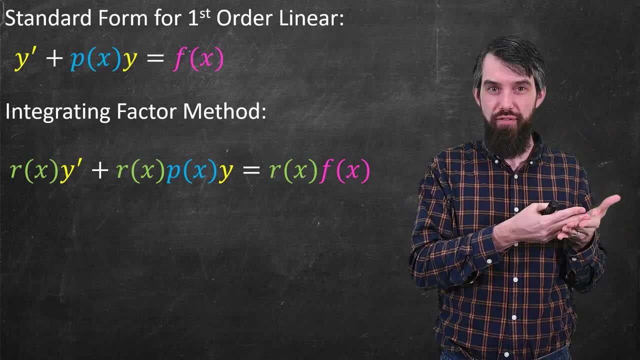 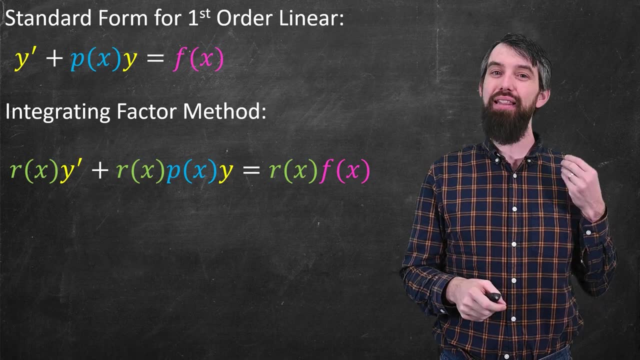 both sides of an equation by some non-zero function, r of x. Now what I would like to do- and I can't yet do it, but what I want to be able to do- is take that left-hand side and just rewrite it as the derivative of something perhaps. 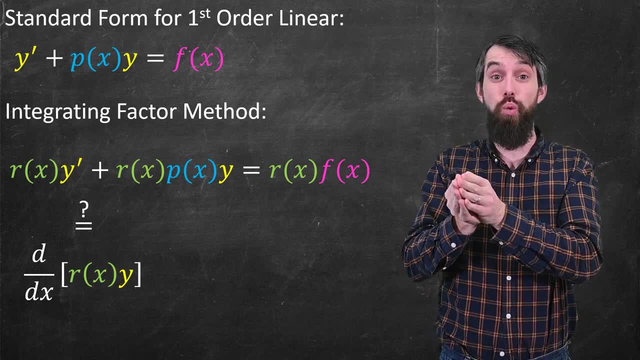 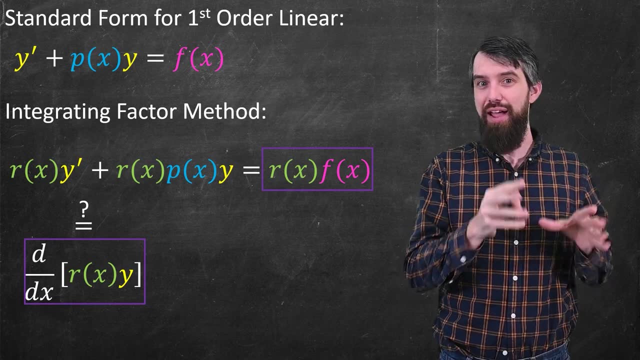 the derivative of the integrating factor r of x multiplied by y. And the reason that I would like to be able to do that is if I had, then on the left-hand side I'd have a derivative, on the right-hand side I'd have a function of x and I could. 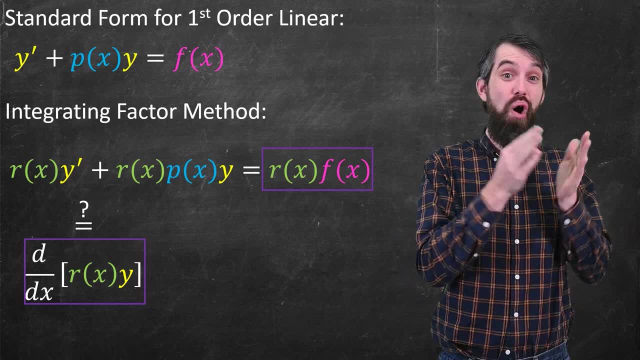 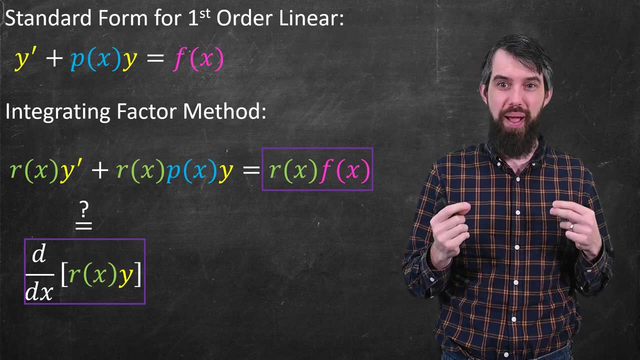 just integrate both sides. with respect to x, That would tell me my r times y divide up by r and that would tell me my y. So I would love if I could write that left-hand side in this format as the derivative of r of x times y of x. But I mean it doesn't. 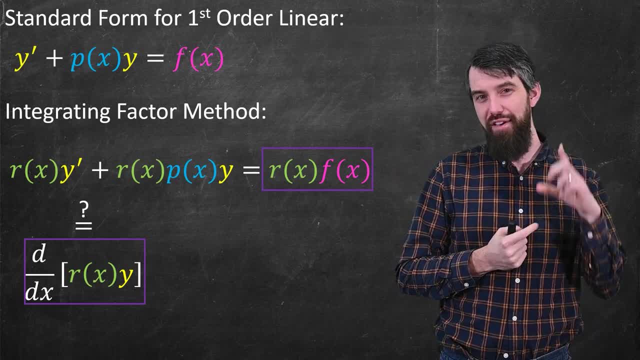 at all. look like that right now. Well, what if I take the derivative of r of x times y of x? Well, what if I take the derivative of r of x brothers? then I should get a product identity prior to x. is that right? 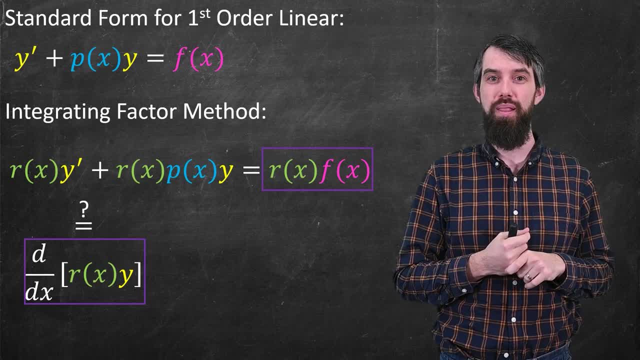 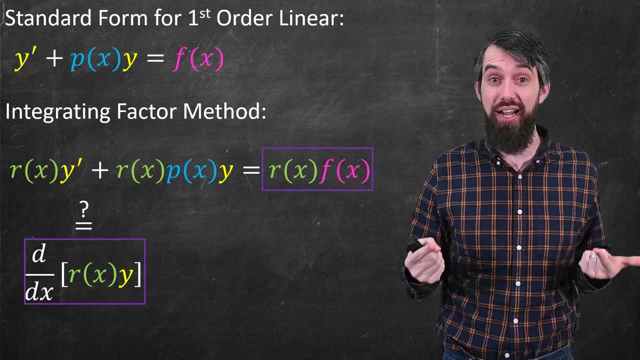 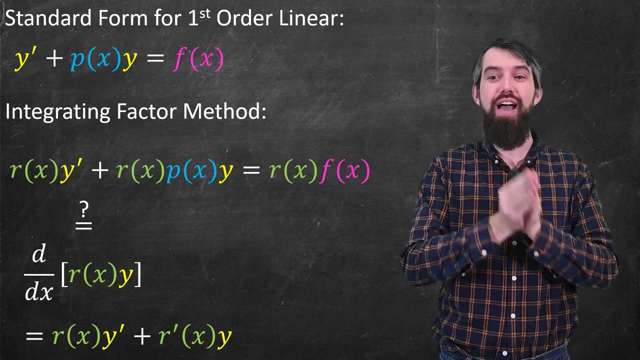 When I take the derivative of y and I wrote all the product knee, I would have a product value which is the same as the derivative of x times y of x And that would draw out r of x times y, prime plus r of the restaurants with n plus r of x times y. 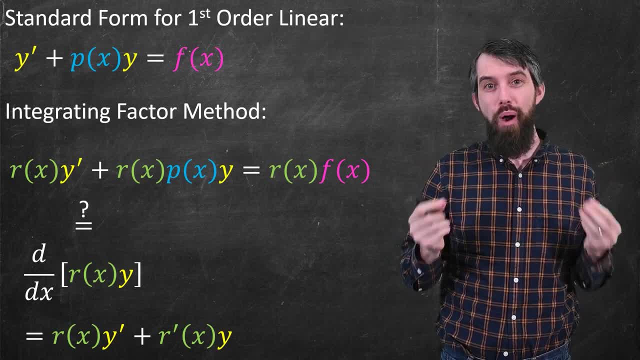 So see, if I take the derivative of y, I'd have the product value of x, and by adding up the product that would come to a derivative of x, And that's the yesterday's product rule. So I'd like to simply büyükly fragment the. 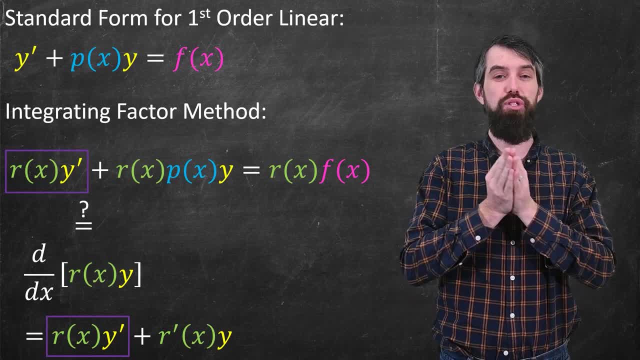 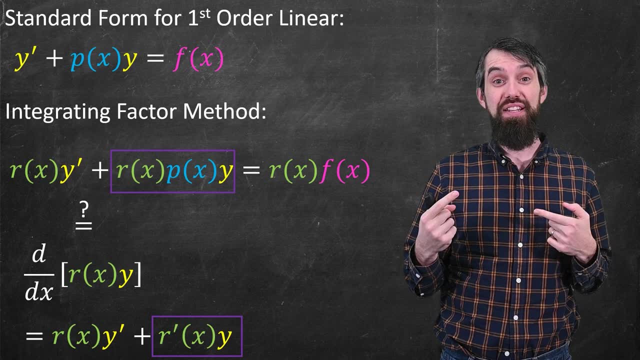 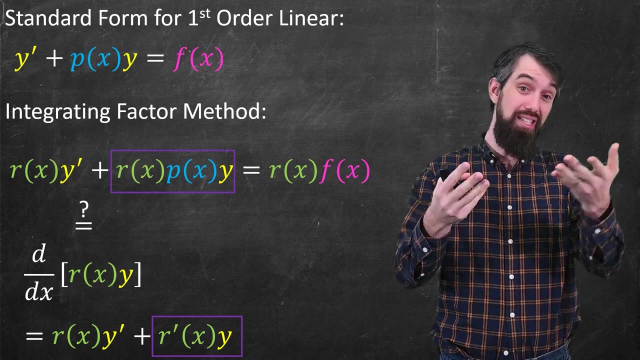 there's a first term that's identical for both of them: the r times, the y prime. That's the same. Okay, looking pretty good. But the second term is quite different. In what I have it's r times, p times y. What I want it to be, it's r prime times y. At least there's a y in both, so I could. 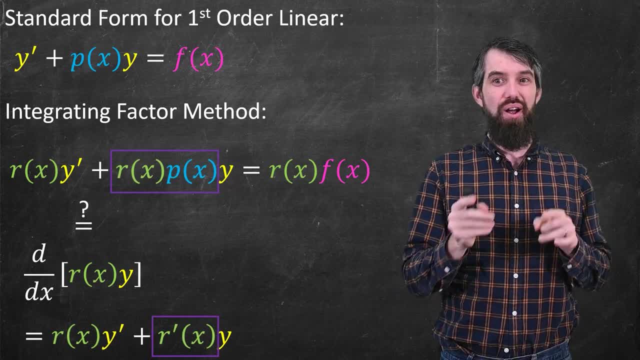 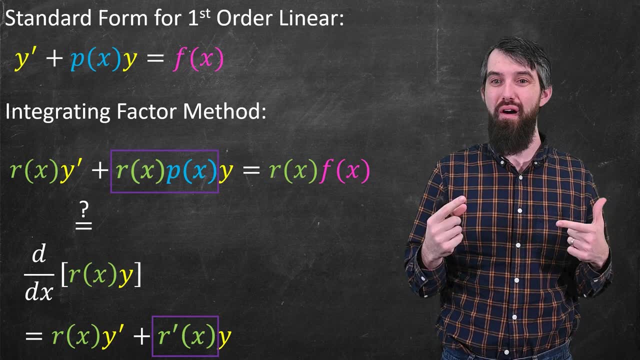 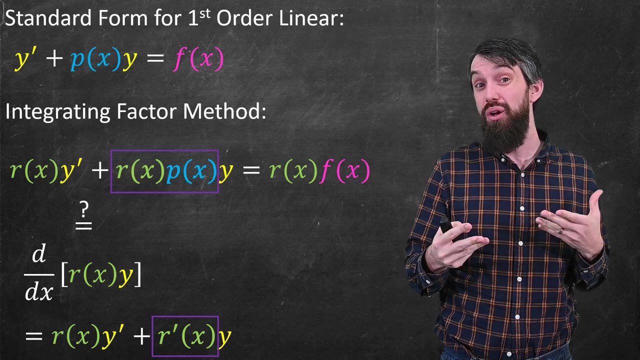 actually just get rid of the y. in my comparison It's saying r times p would have to be equal to r prime. So again I'm just trying to find a function of r of x that would work out to make it nice the way I want it to be. And if that was to be the case, then these two things would have. 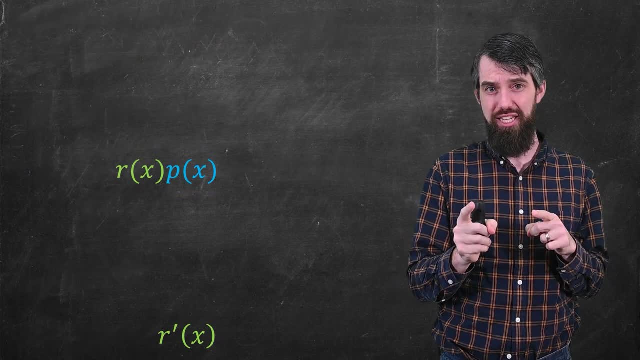 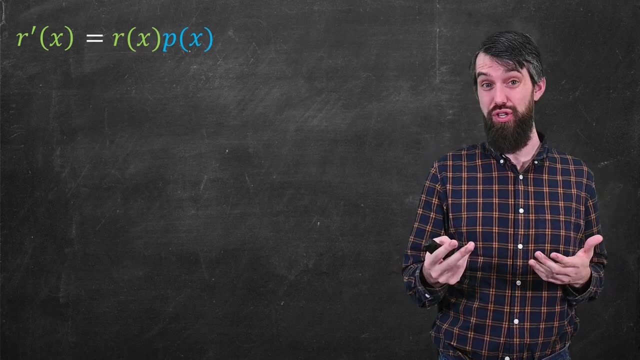 to be equal. Okay, so let's just play around with that. Let's just set those two things being equal and just see what we get. This here is a differential equation- It's actually a first order differential equation in the variables r and x. Okay, in fact, I can do more than that. 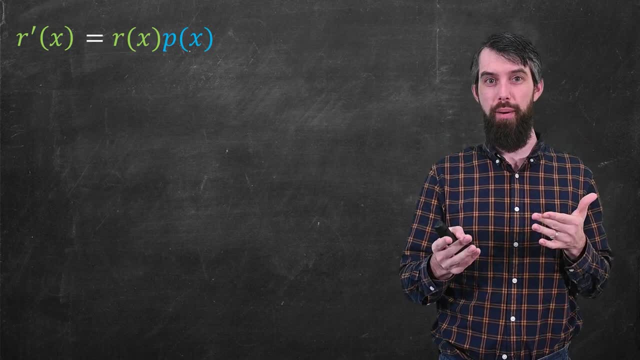 It's not only just a first order, it's a separable first order. So let me just go and separate it using the method of separation of variables. I'm going to divide out by the r of x on both sides and then I'm. 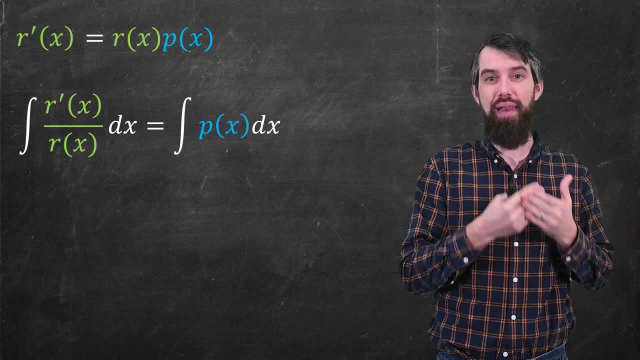 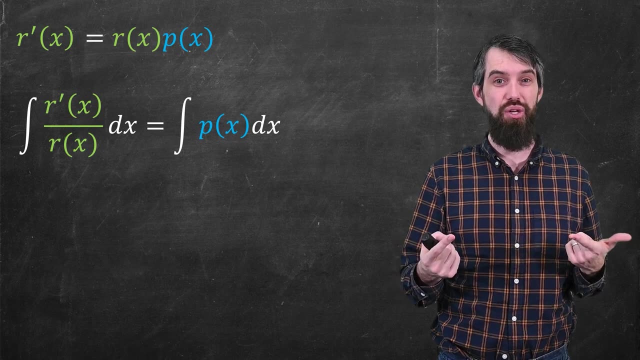 going to integrate with respect to x on both sides. So I get r prime over r on the left and then the integral of p of x on the right. So now I'm solving some interval. Well, the left-hand side, I can do. It's going to be a logarithm. If my r of x is positive, I'll say more about that. 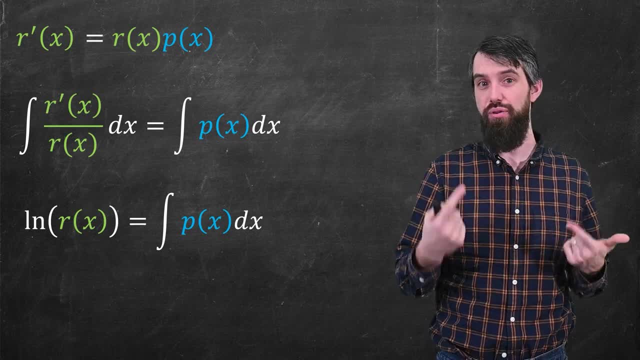 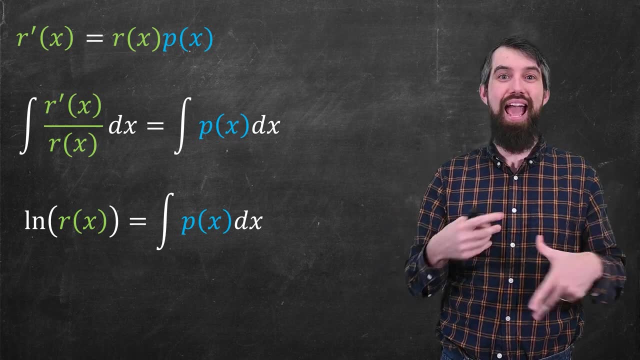 in a second. then it would be: the logarithm of r of x is equal to the integral of p of x. Now I don't have a p because I'm doing a general example right now, so I can't evaluate the right-hand. 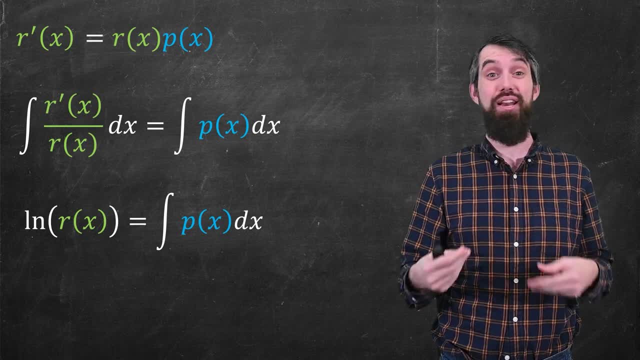 side. I'll just leave the right-hand side as the integral of p of x dx. If you had a specific p of x, you could go and do this, But regardless, I have a logarithm. I want to get rid of that. 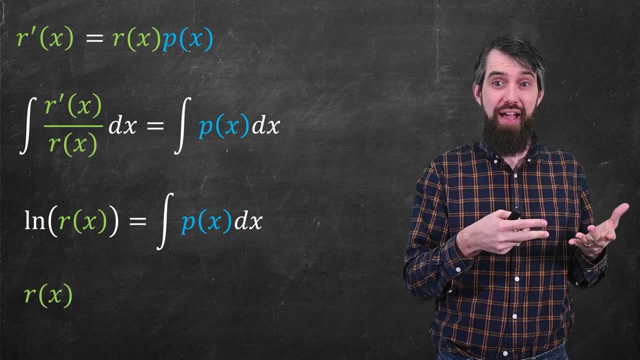 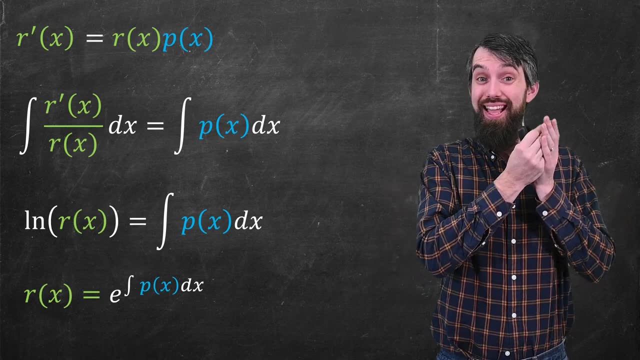 logarithm, I'm going to take an exponential, And so my r of x is e to the integral of p of x, dx. So this is an answer. This tells me what the integrating factor is that I should choose. It's that function. Take your p of x. 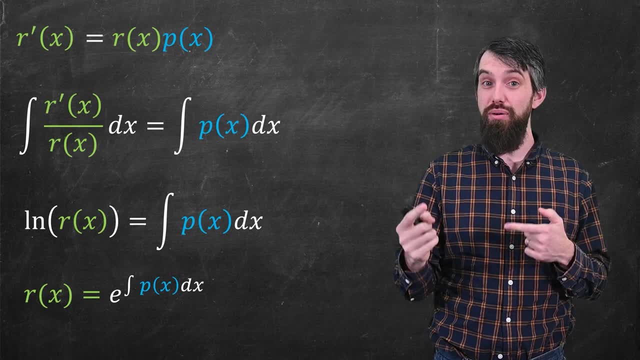 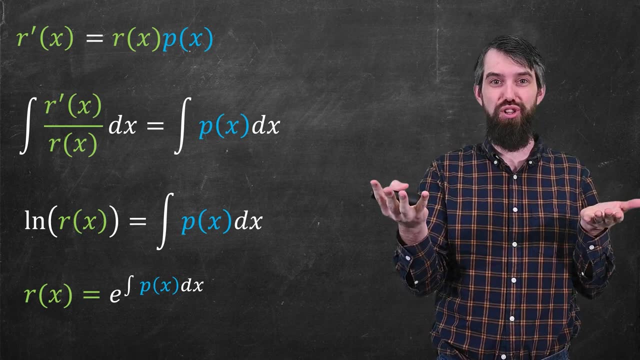 Integrate it. It's e to whatever. you get Two little notes here. First of all, I could have chosen this to be negative as well. It wouldn't matter though. I mean I was multiplying every single term of my differential equation. 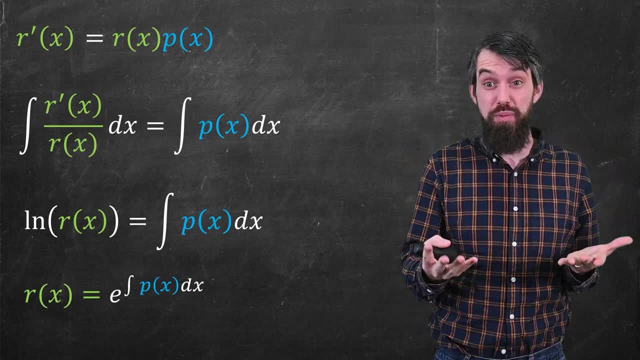 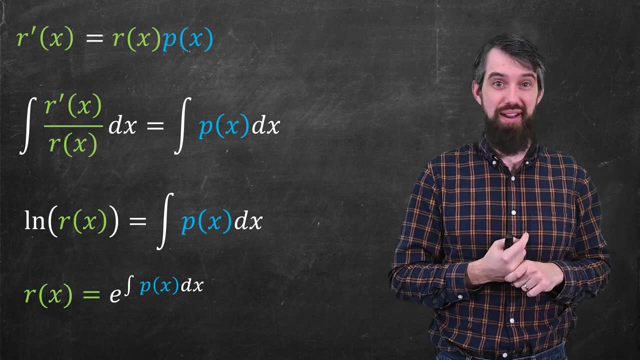 If I multiplied it by a negative or positive, it doesn't matter, I'll just assume it's positive. Second thing: when you do an interval, well, you get a constant of integration. that should come out of that, But I don't care about the constant. Again, I'm trying to find some r. 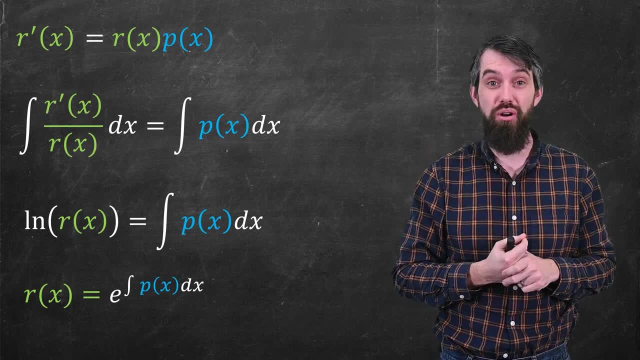 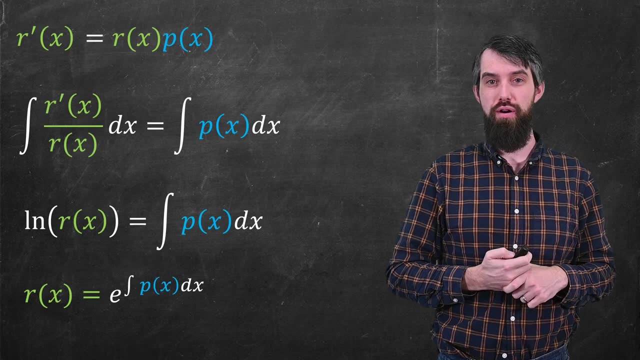 of x that satisfies my property. Well, I'll just choose c equal to 0, so I don't have to think about the constant. As long as it works, it works Nevertheless. here it is. I have my r of x. 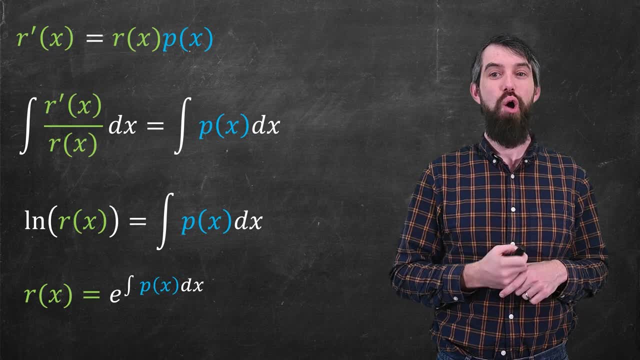 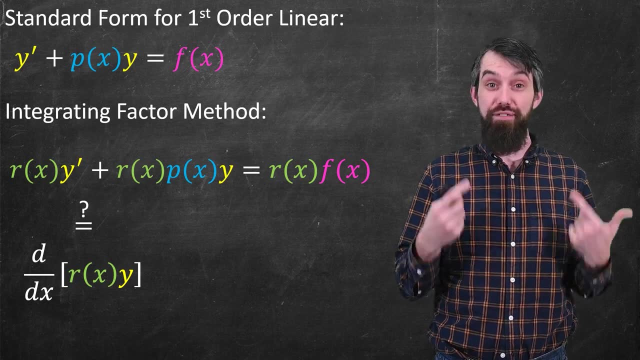 OK, so let me go back just a moment to remind myself of what it was that I was talking about. This was the previous slide we'd compared a few minutes ago, And what we were saying was: we wanted to find an r of x such that we could have this nice thing that we understood. 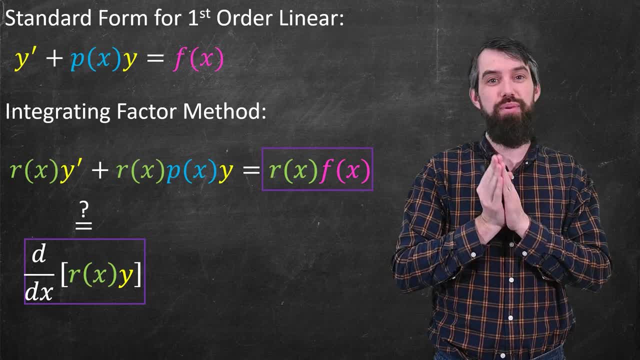 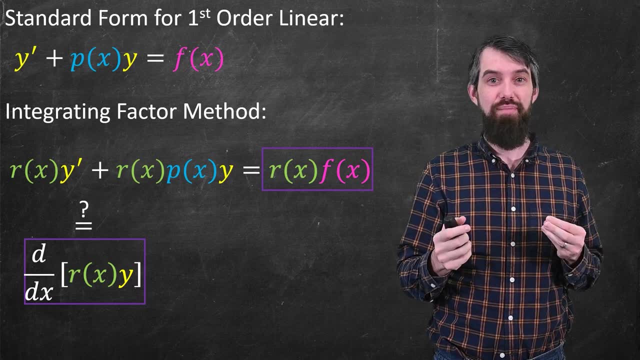 The derivative of r of x times y on the left-hand side was set to be just some functions of x on the right: r of x times f of x. So that's what I'm hoping to get, And indeed I found an r of x such that this is going to be true. 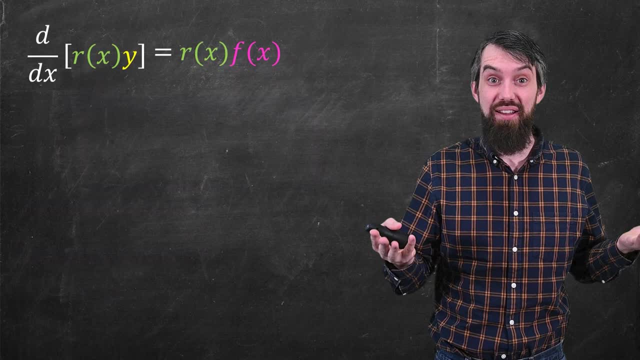 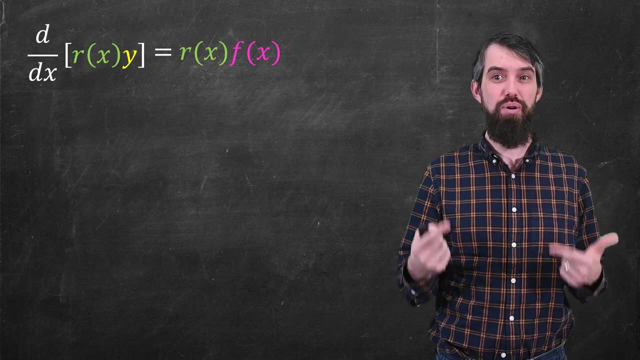 So now, I actually want to solve this equation. Well, I can do that. It's just a derivative on the left, Indeed, that was the whole point. I can now just integrate this. So what do I get? Well, integrate both sides, and so you get an integral of r of x times. 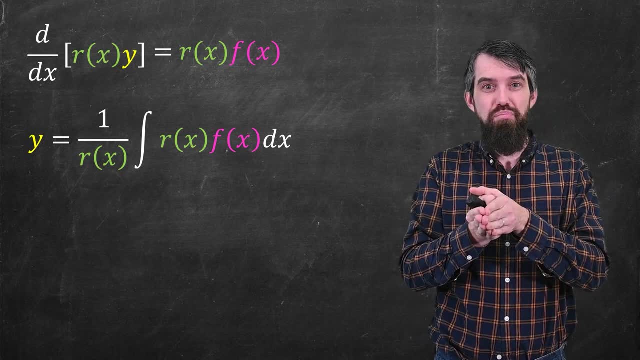 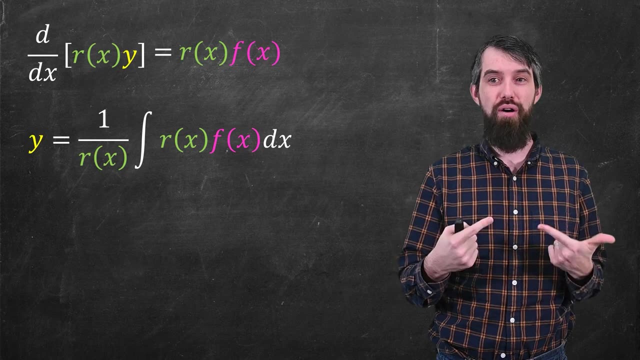 f of x. On the left it was r of x times y, so I need to divide out by the r of x. Final answer: y is 1 over the r of x and then the integral of r of x times f of x. 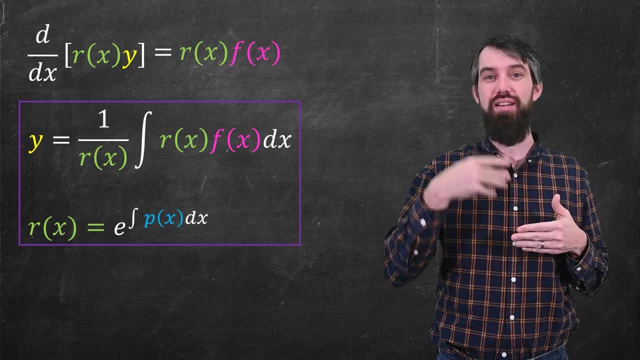 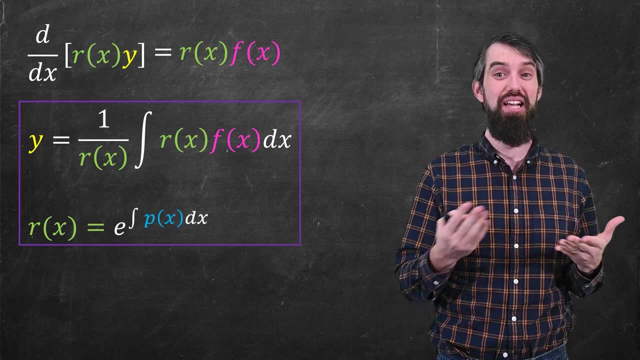 where that r of x is the thing we computed previously, e to the integral of the p of x, dx, And that's my answer. By the way, one little thing: I've noticed on tests that, for whatever reason, students often forget the 1 over r of x factor. they do everything else correctly, so just make. 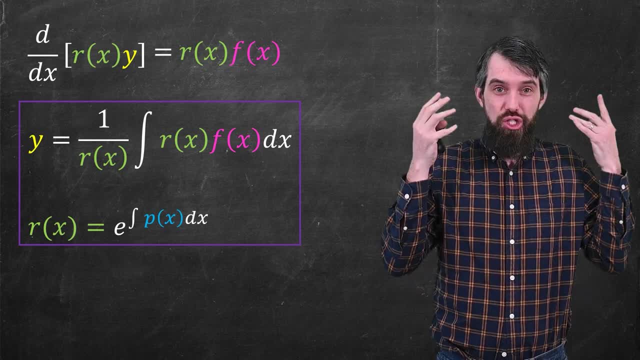 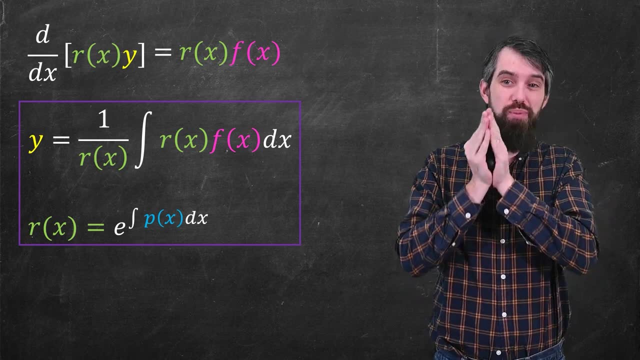 sure that's not going to be you. Either way, what we have is a solution to the original differential equation. Indeed, I encourage you to verify this by taking the derivative, plugging it in and making sure that you get whatever you get. 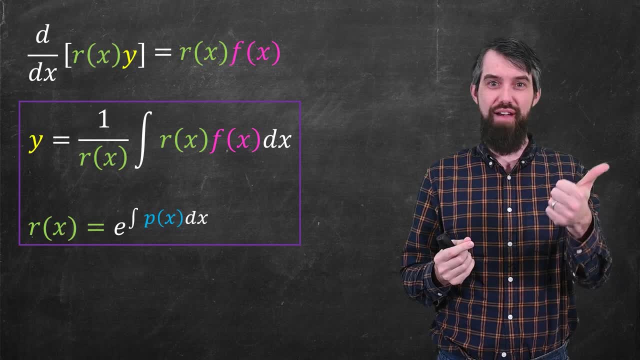 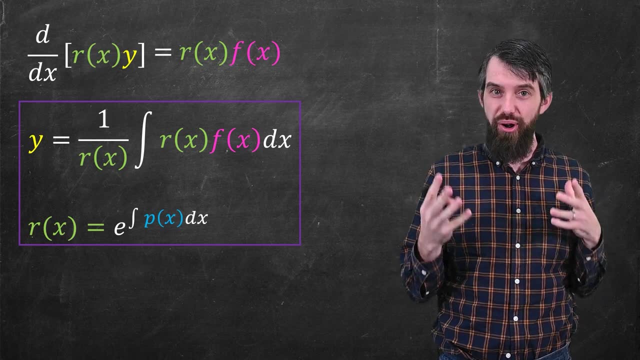 Now I owe you a concrete example of this, where I tell you the f of x and tell you the p of x and we go and compute it out. I will do that in the next video, But while we're still in the slightly more general and abstract sense, I want to focus. 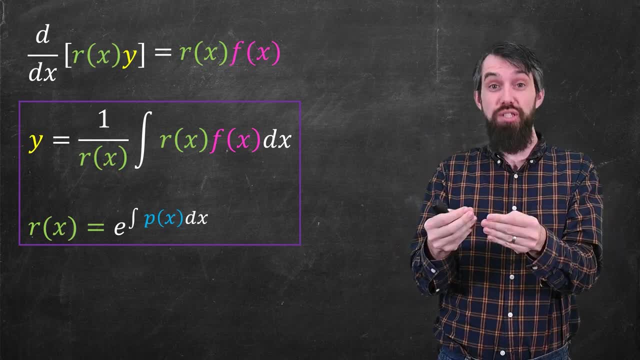 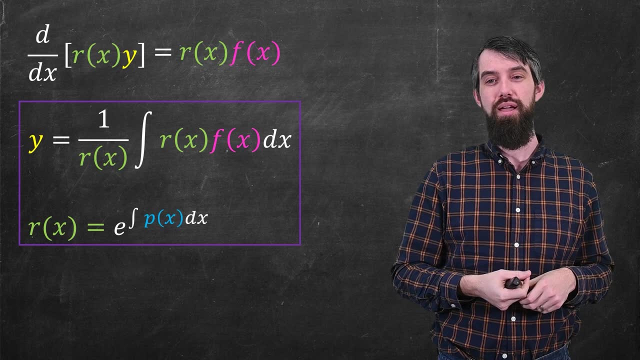 a little bit on what the existence and uniqueness consequences are when you have this solution and use this methodology to solve a first-order linear differential equation, Because the first thing I want to note is, when I look at this, there's two intervals here. 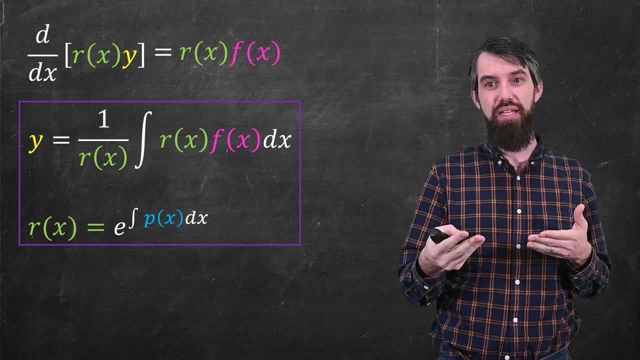 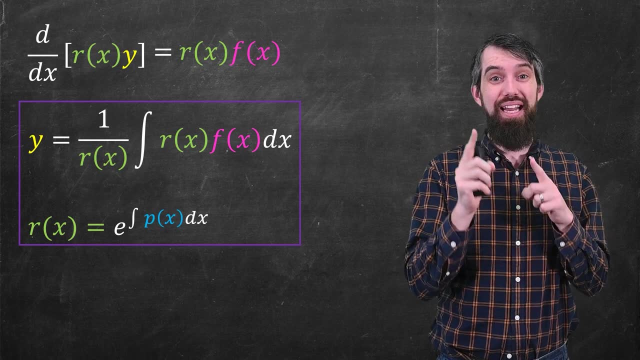 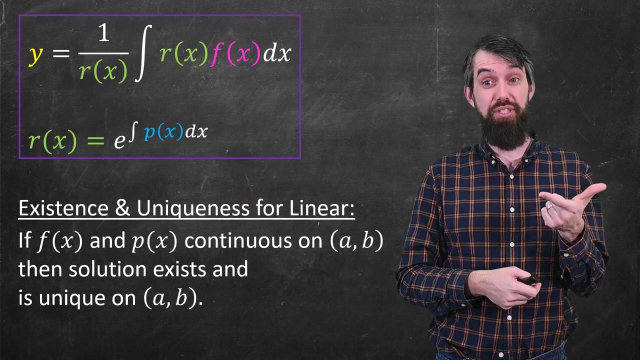 The integral of p of x And then the integral of r of x times dx. So as long as you can do those intervals, you get a solution. That is, I have the following existence and uniqueness theorem. It says that if f of x and p of x are continuous, which is sufficient for me to be able to integrate-